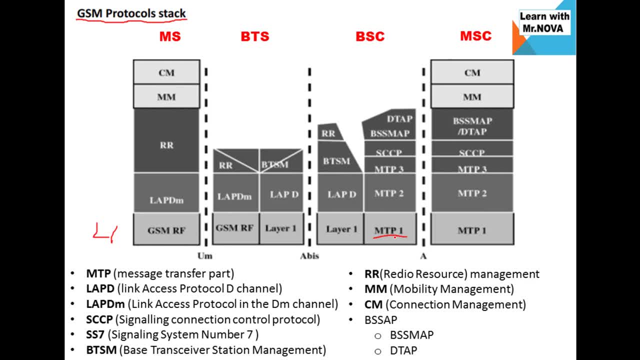 version 1, version 2 and version 3.. so message transfer path, basically, is a layer one protocol that allows media files to be transferred automatically to and from mobile devices. there are one protocol that allow messages that allow you to access your texts, media files, to be transferred automatically to and from mobile devices. okay, and the second. 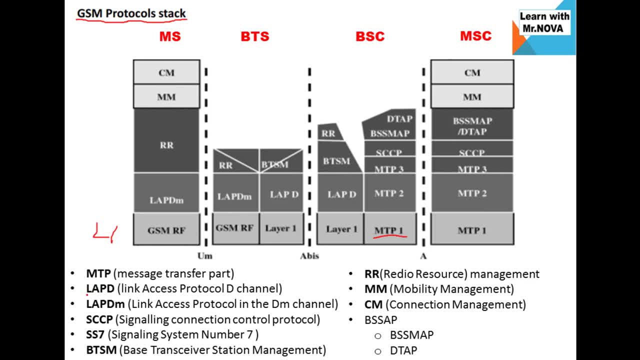 protocol I'm going to proceed with is the link access protocol, the channel. you know the link access protocol, the channel is an integrated service digital network, that is I, integrated service digital network. it's an integrated service digital network protocol providing error-free transmission between the base, the base station controller and the Mobile. 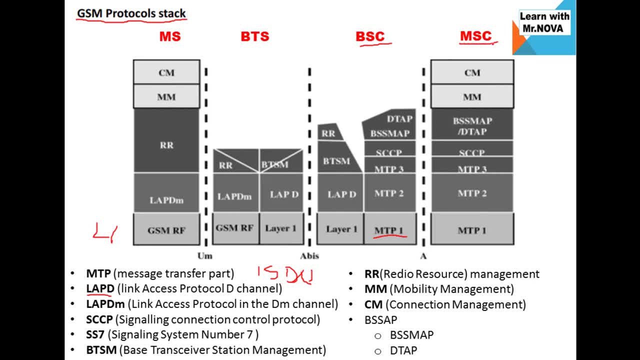 Switching Center. so I will repeat that the link SS protocol, the channel, is an integrated service digital network protocol providing error-free transmission between the base station controller and the mobile switching center. the next protocol is the link access protocol in the gm channel. it is a modified version of the link access protocol. it's a modified version of the link. 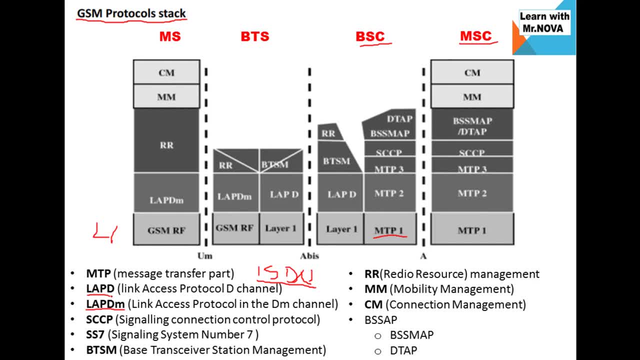 access protocol. it is used in gsm to support the transport of information between the mobile and the network. so the link access protocol in the dm channel is used in a gsm to support the transfer of information between the mobile and the network. so that's the role of this protocol. 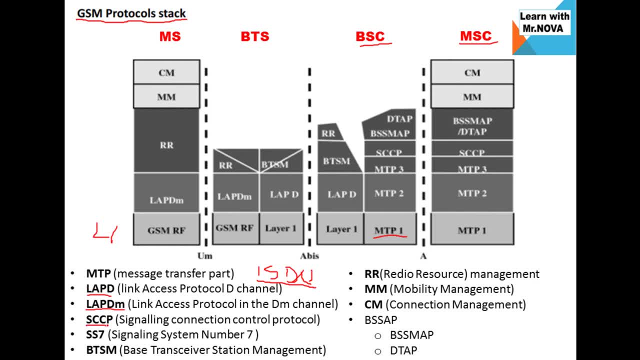 the next protocol we have here is the signaling connection control protocol. now, the signaling connection control protocol is basically A network layer protocol that provides extended routing flow control, segmentation and connection orientation. I will repeat that a signaling connection control protocol is a protocol that provides 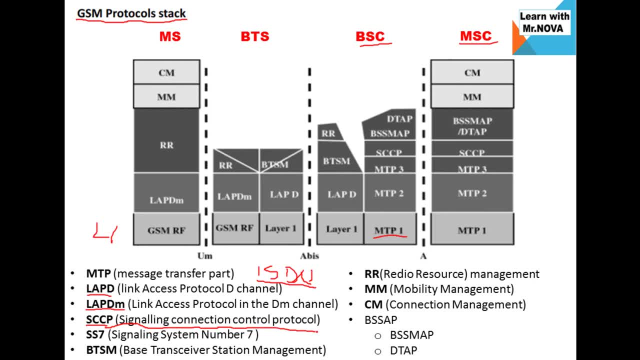 extended routing, flow control, segmentation and connection orientation. I believe in some videos in the future, I'm going to clearly explain some of these protocols in details. So, since this video is just a summary of the GSM protocol stack, so I'll just move straight. 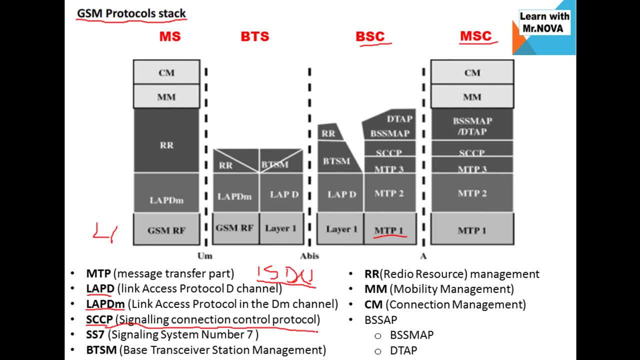 to the point, given the role of the protocol. Okay, the next protocol we have here is a signaling system, number seven. Now, this protocol is used for signaling between the mobile switching center and the base station controller. You know, the signaling system number seven is used between the mobile switching center. 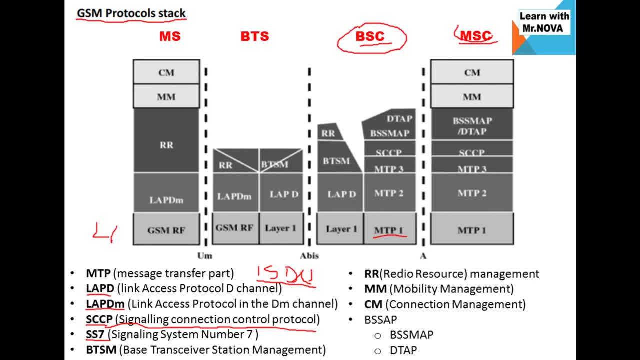 and the base station controller. This protocol also provides uh also uh transfer all management information between the mobile switching center and uh. you have uh the: the, the home location register, the visited location register, the authentication center, the identity equipment identity register. 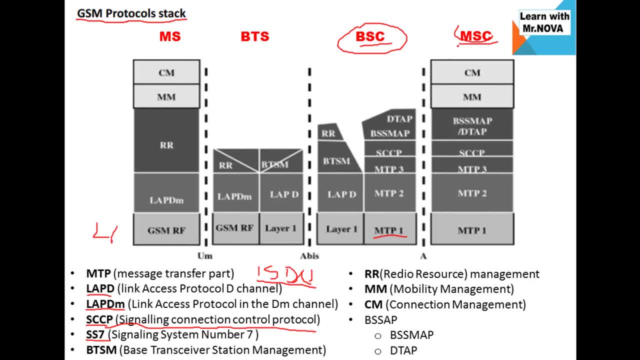 You know, when you Draw the, the GSM uh architecture, you get to know the, the, the, the visited location register, the home, the home location uh register, and many more. So, in a nutshell, the protocol is used for the transfer of management, management information. 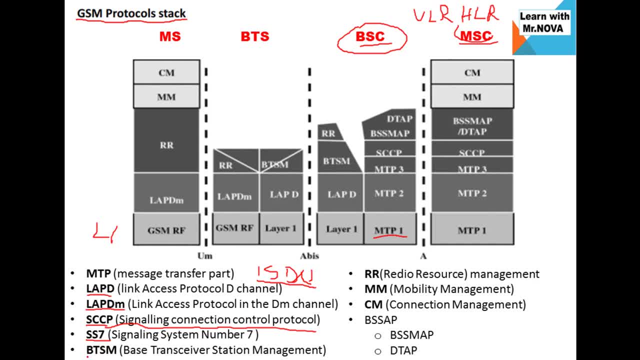 Okay, Okay. So the next protocol we have here is a base transceiver station management, which is abbreviated BTSM. You can find it here. This is the base transceiver station management. Now, the base transceiver station management is responsible for the transfer of radio resource. 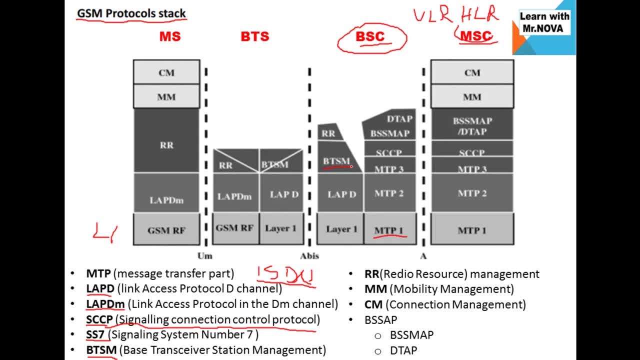 information to the base station controller. Responsible for the transfer of the radio resource information to the base station controller. Okay, Okay, Okay, So the base station controller. The next protocol we have here is the radio. Sorry, This is a. this is a radio. 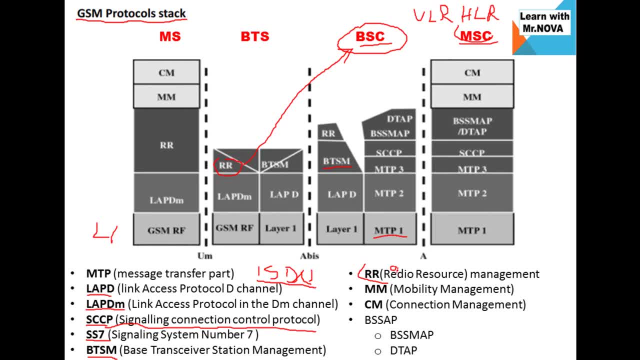 It's letter a, not E. Okay, The radio resource management you know are the third layer. This is a third, this is a layer three. layer three of the GSM protocol is divided into three sub layers. have the radio resource management. we have the mobility management and the connection. 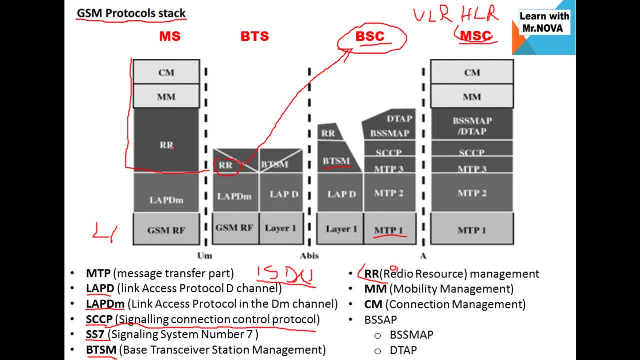 management. so i'm going to begin with the radio resource management. so the radio resource management: it is in charge of establishing and maintaining a stable, uninterruptible uh communication path between the base station controller and the mobile and the mobile station. so the radio resource management is, i will repeat, that is in: 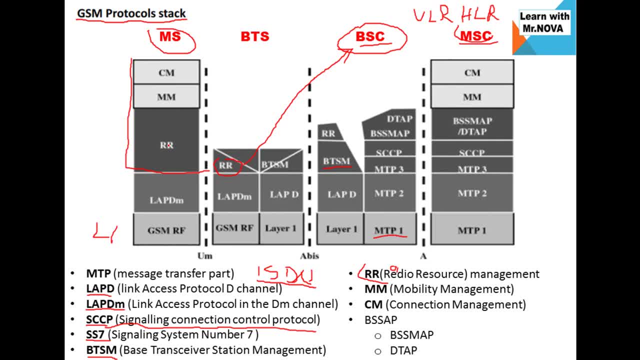 charge of establishing and maintaining a stable, uninterrupted communication path between the mobile station and the mobile switching center, over which signaling and user data can be covered. you know, the radio resource management is directly below the mobility or management or layer. so the next we have here is the mobility. 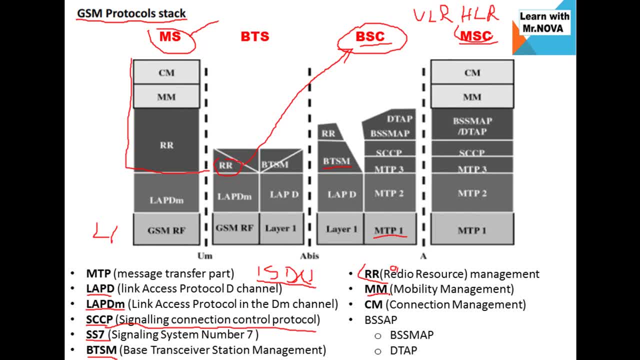 management. now, the mobility management is stacked directly, uh, above the radio resource management. as you can find on the diagram. it handles the function that arises from the mobility of subscribers, as well as authentication and the security aspects. so i'll repeat that the mobility management- it handles the mobility of subscribers as well. 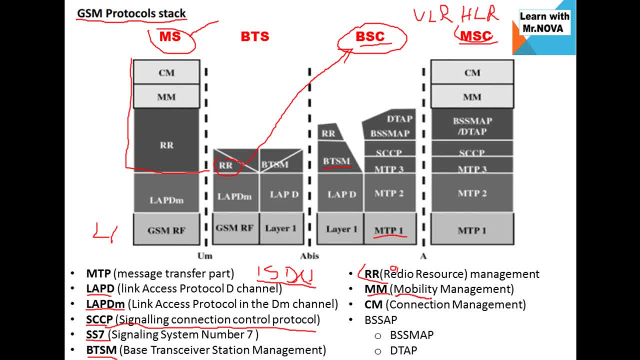 as authentication and the security aspects. okay, and the last layer we have here is the connection management. you know, the connection management is generally, it handles general call control. uh, it manages some supplementary or services and short message services. i'll repeat that, the connection management, it handles general call control. 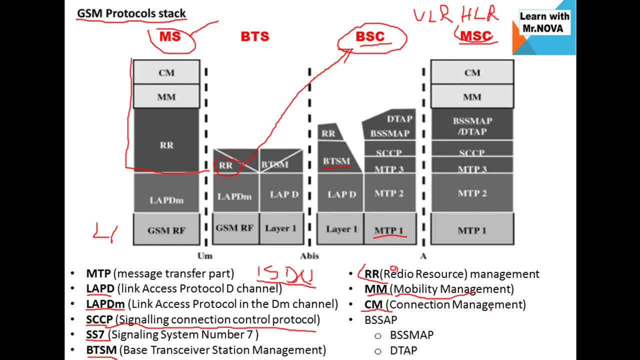 it manages supplementary services and short message service, which is abbreviated sms. so this is the connection management layer, not forgetting the protocol b, s, s, a p, which stands for base station system application path. now, the base station system application path is a layer 3 protocol. you know the base station. 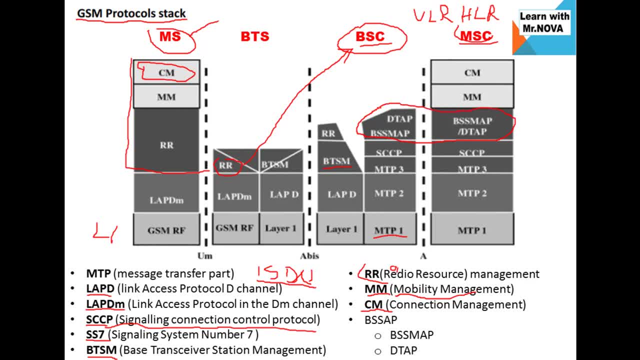 the base station system application path. b, s, s, a p base station system application path is divided into two. it's split it into two: the base station and the data transfer application path. excuse so. So this protocol basically is a layer 3 protocol and the role of the base station system management. 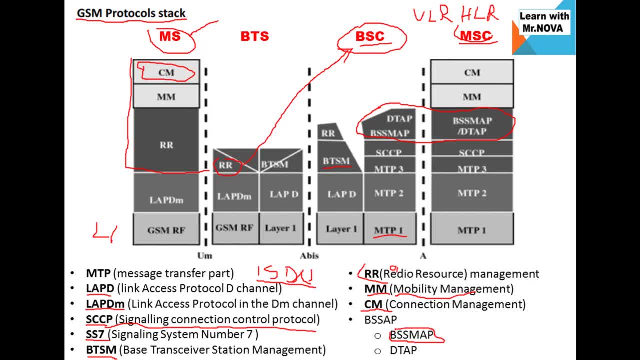 application path is basically used for carrying messages that are not transparent, are not transparent to the base station controller and also supports the procedures between the mobile switching center and the base and the base station subsystem. You know basically to. in order to understand this, you equally need to have an idea of the 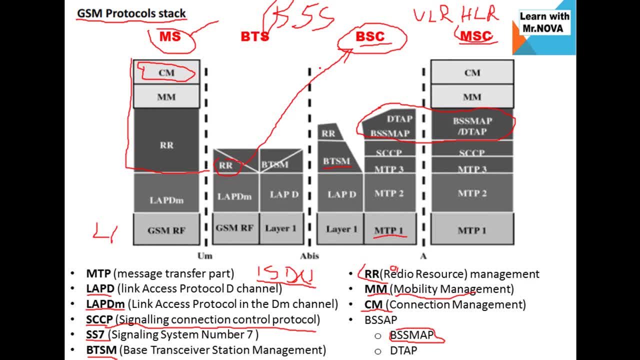 simplified architecture of the GSM protocol stack. So I believe basically these are the main protocols in the GSM protocol stack: The message transfer path, the link as the access protocol, The channel. We have the link access protocol in the GSM channel, which is just simply a modified version. 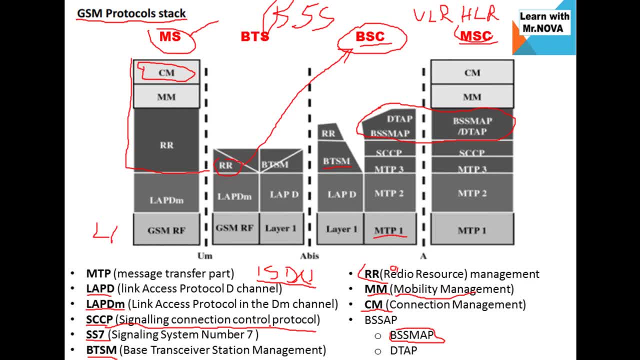 of this. We have the signaling connection control protocol. We have the signaling system number 7.. We have the base transceiver station management. You have the radio resource management. We have the modability management, the connection management. We equally have the base system- sorry, the base station system application path, which. 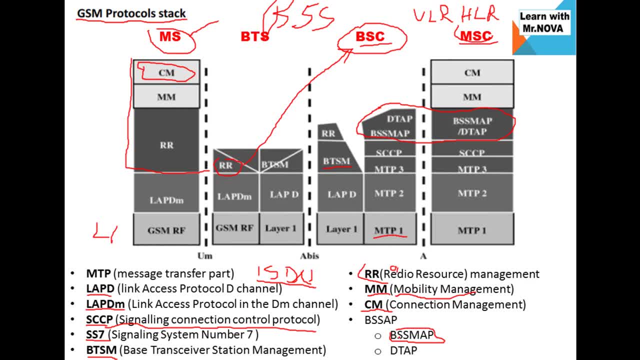 is split into two: The base station system management application path and the data transfer application path. So I hope that you enjoyed this video and if you haven't subscribed at the beginning, please kindly subscribe to promote this channel and to equally click on the notification icon. 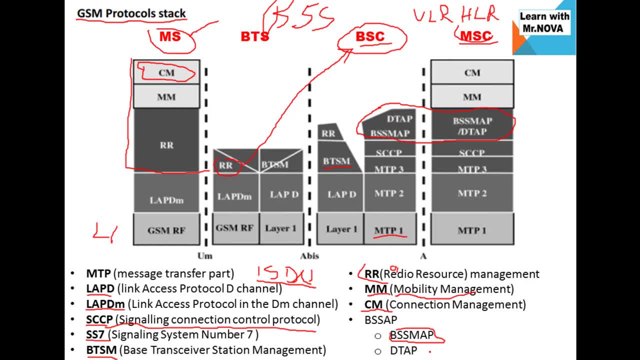 to get notified whenever a video is uploaded on YouTube. So thanks and see you in my next video.